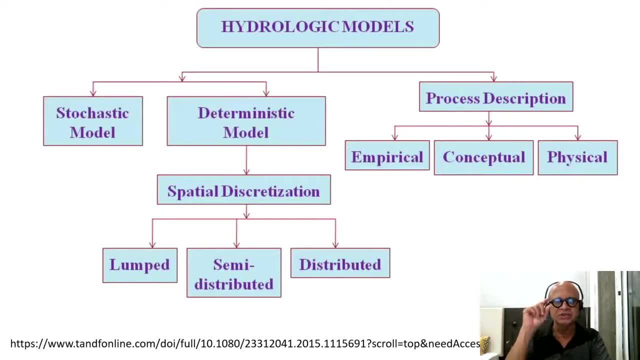 information, Input, output, precipitation storage, soil, moisture, groundwater and runoff, etc. and semi distributed and distributed. so I won't go into the details, but you can see what that means. they can be split into hydrological resource units or just grid points, where each grid point 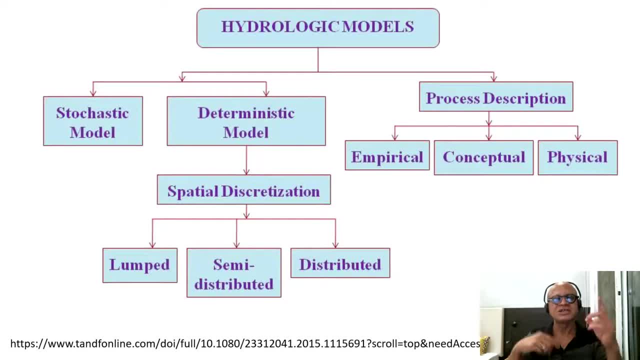 is doing: water balance, energy balance, exchange with the atmosphere, percolation, runoff and so on and so forth. And some models focus on process descriptions, which could be empirical. so let's say how a stream flow is created over a watershed. could be conceptual, could be physical and 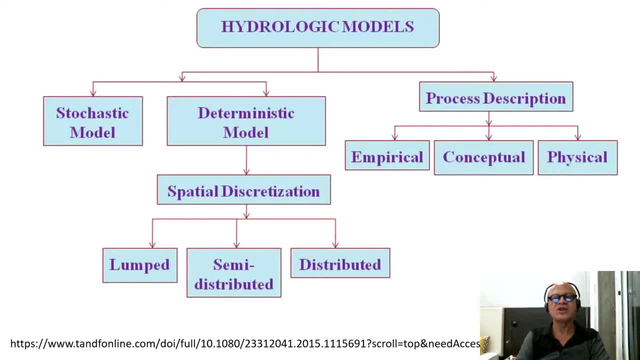 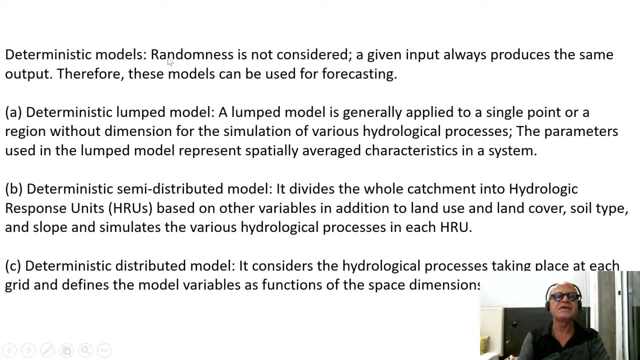 so on. so I'm again not going to go into great details, but looking briefly at what we mean by deterministic models. Here randomness is not considered, So even the precipitation itself could be a random forcing. a given input always produces the same output, so it's deterministic. there is no stochasticity to it. of course that doesn't. 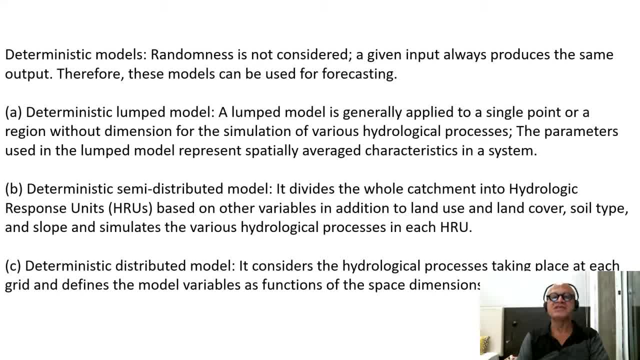 mean it's completely always producing exactly the same number, because the nonlinearities in the system itself can produce sensitivities to initial conditions and so on. Therefore, these models can be used for forecasting. Deterministic lumped model. a lumped model is generally applied to a single point or 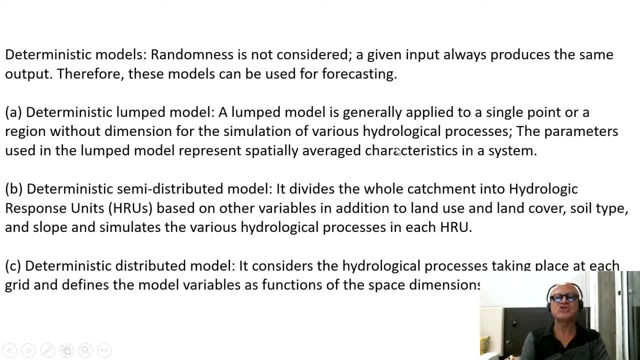 a region without dimension for the simulation of various hydrological processes, So the parameters used in this lump models typically represent spatially average characteristics in a system, So it could be average soil properties, averaged amount of rain, average temperature, average water demand, and so on. 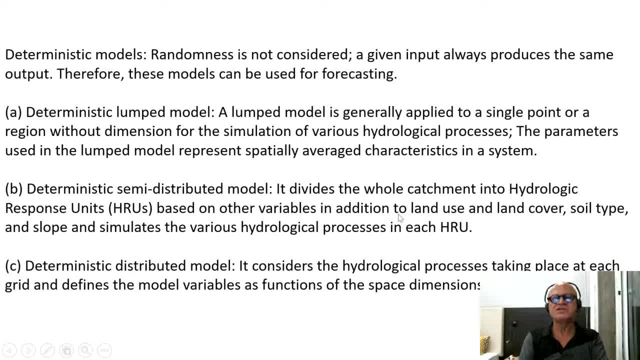 Whereas deterministic semi-distributed models are generally applied to a single point or a region without dimension for the simulation of various hydrological processes, The semi-distributed model divides the whole catchment into hydrological response unit based on other variables in addition to land use and land cover. 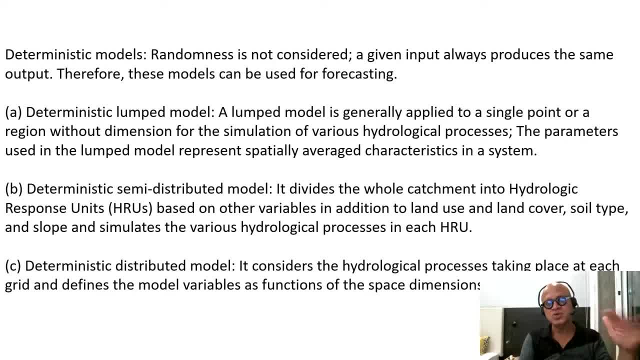 So what kind of vegetation, agriculture, urban, rural, land cover. there is Soil types and slopes, So how the water flow is affected by the slopes, and it simulates the various hydrological processes in each H2O model. So that's what it is. 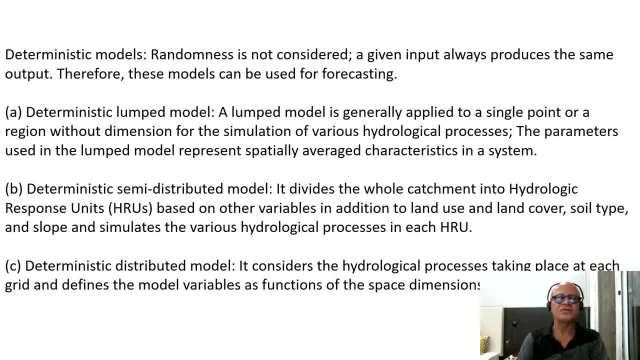 H2O is the hydrologic response unit and then each unit is related to the next unit for water balance. So weather is forcing from the top, water that falls is flowing through the hydrologic response unit. Sorry about that. So deterministic distributed model considers hydrological processes taking place at each. 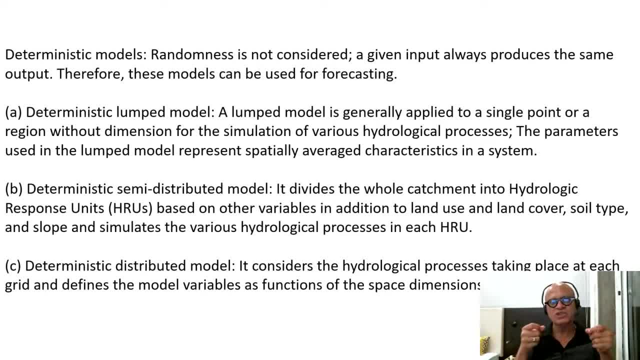 grid point. So if you have a watershed, You cover it with, let's say, 10m x 10m grid, 100m x 100m grid or whatever, depending on the computational demands and resources. and it defines the model variables as functions. 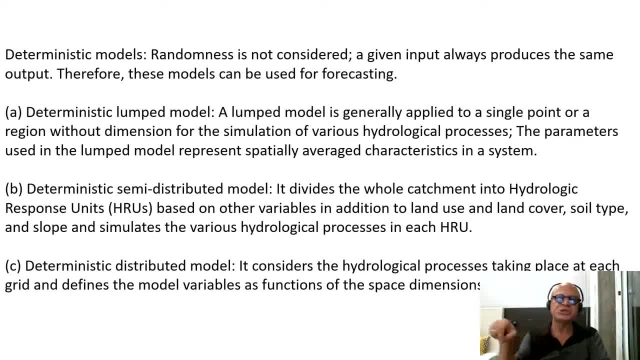 of space dimensions, So at each longitude and latitude, for example, it resolves all the processes of energy exchange, water exchange, water seeping through, water flowing out, water coming in. These are critical, But what are they essentially trying to do? 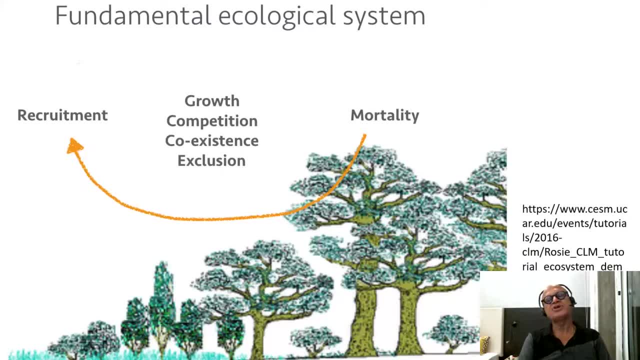 You cannot just do hydrology anymore without worrying about the entities, other parts of the ecosystem that are part of the storage, evaporation, evapotranspiration and so on. So now people are moving more and more So here, for example when we say land use and land cover. 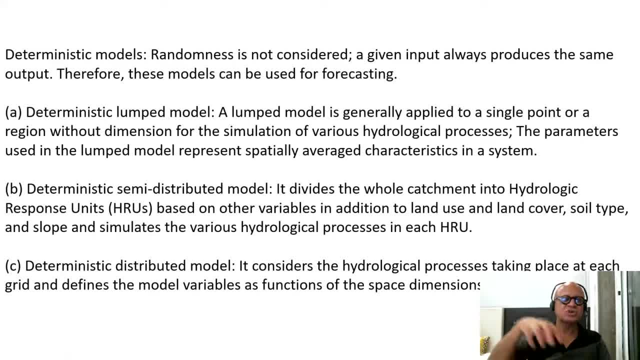 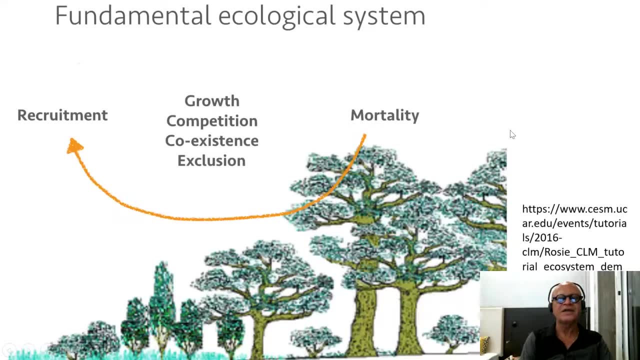 You can just prescribe the land use types. You can say agriculture, forest, grassland, bare land and so on, And each will have some properties like hydraulic conductivity and so on. But when you do these things, you include interactive ecological response as well. 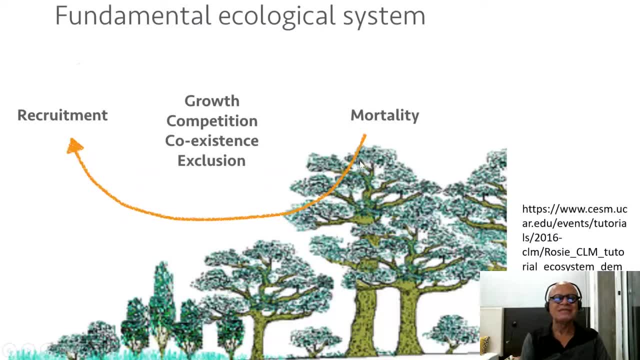 So ecological models are basically trying to do: mortality, growth, competition, coexistence and exclusion. So how the ecosystem determines its composition. there are ideas about whether each ecosystem is optimized for production, for resilience, for biodiversity and so on, But nonetheless, recruitment is essentially for each seed that is thrown. how many survive? 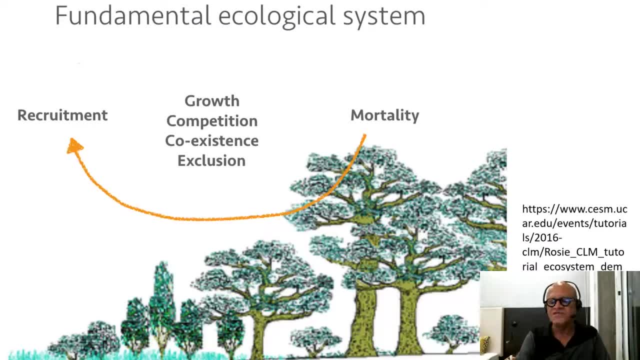 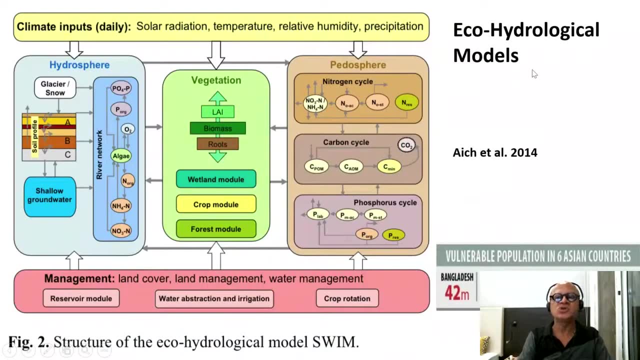 to grow up to be adults. That's kind of a loose. it's actually a pretty good definition, OK, So now we have what are called eco-hydrological models. So I'll just show one schematic from this model called SWIM, which takes climate inputs. 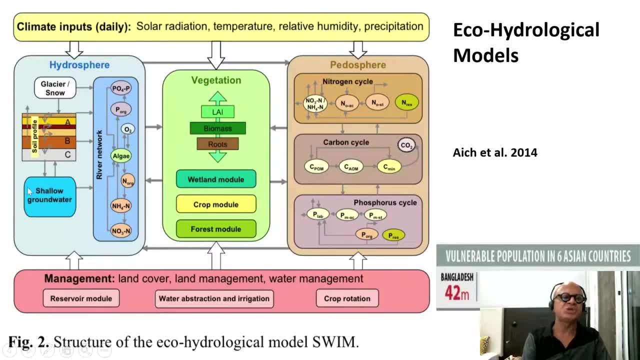 daily solar radiation, temperature, relative humidity and precipitation. It has a hydrosphere with various components like glacier flow, soil profiles, shallow groundwater and the river network that's supported with it. It also combines management, So land cover, land management, water management. 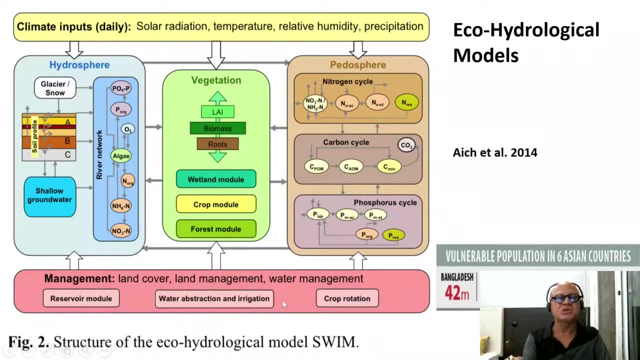 So there is a reservoir model. in it water abstraction, irrigation is modeled and crop rotation is modeled and so on. These are not easy to do. Water abstraction and irrigation data is needed desperately, let's say at daily time scale, to do these sorts of models. 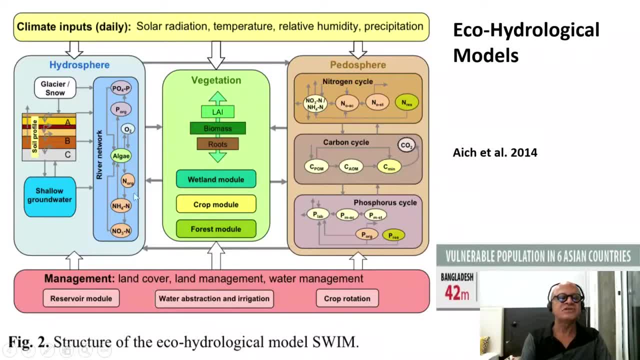 But it's not always available. And you can see that this one is even doing some biology, OK, With algae and phosphorus nitrate, ammonium and so on, nitrogen oxygen. So it's doing ecosystem as well, And obviously they have a vegetation module because it's an eco-hydrological model. 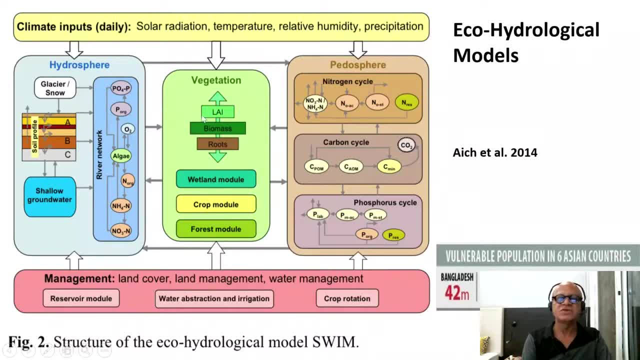 And it has a soil module called a pedosphere. So you can see quickly it gets very complicated but very important. The point always is that this also includes carbon cycle. So carbon storage and carbon exchange with the atmosphere, organic matter flow through the rivers etc are done. 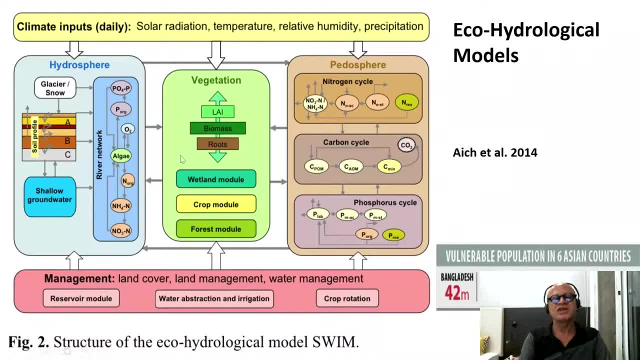 But the uncertainties. that's what critically matters, because there are literally thousands of parameters that go into these, that are based on data, which is very sparse, and process understanding, which is always trying to be improved. OK, So this looked at vulnerable populations in six Asian countries. 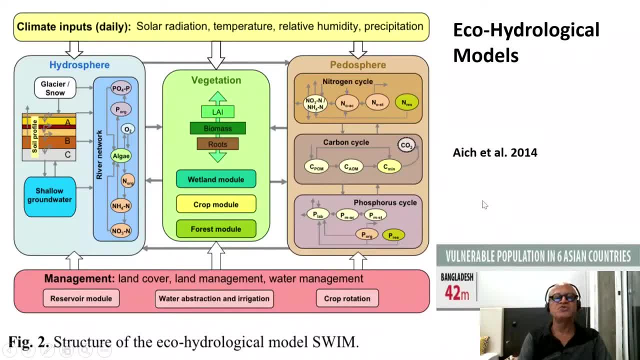 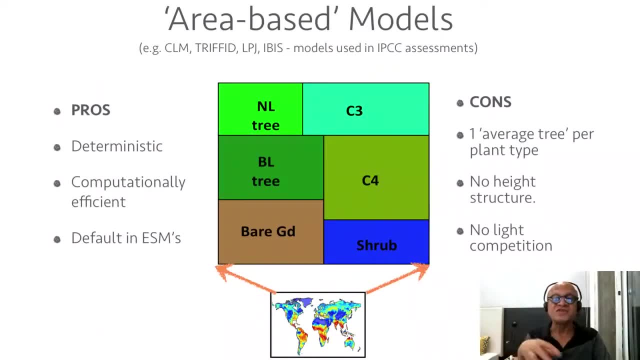 OK, So trying to do this remembering that the hydrologic flows don't observe international boundaries, Rivers cross international boundaries right. So there are area-based ecological models, which the examples are: the Community Land Model, TRIFID, LPGA, IBIS. 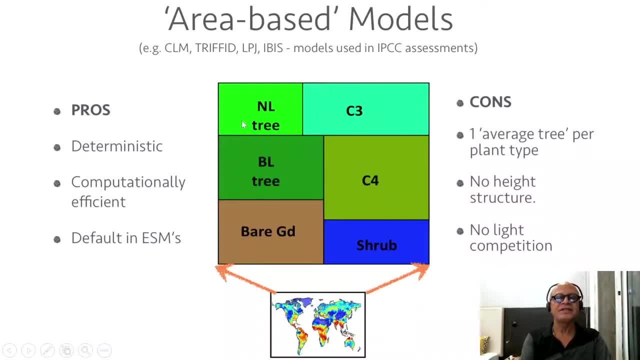 They are used in IPCC assessments And this is like media, And the way that these models can be used to study these different earth forces. is that in the global, global scale? OK, The questions are mostly these. So what? you don't see much of these all the time. 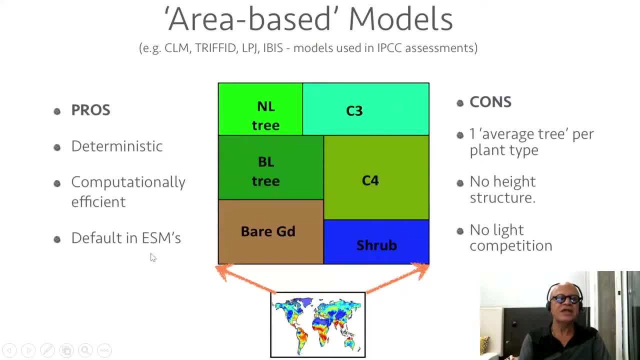 that they are deterministic, they are computationally efficient and they are the default models in earth system models. So they are usually called land models, not so much vegetation or ecological models. The cons are that they are one average tree per plant type, so you have that problem there. 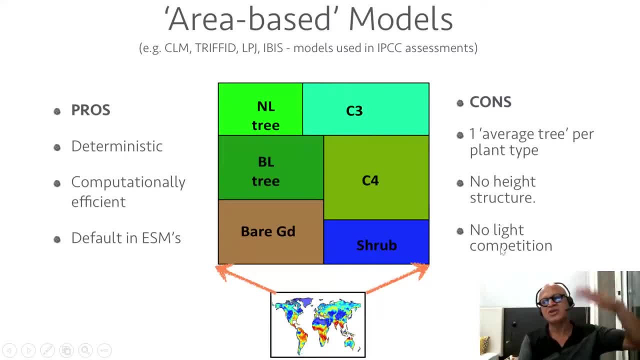 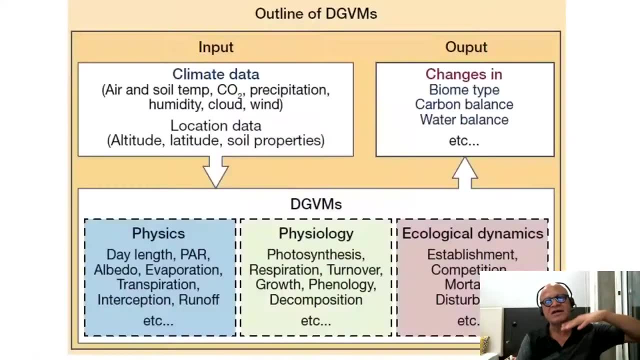 No height structure, so the boundary layer interactions are not well represented and there is no light competition. If you don't have a height, you cannot really add effectively light competition. So the latest approach are called dynamic global vegetation models, which take again. 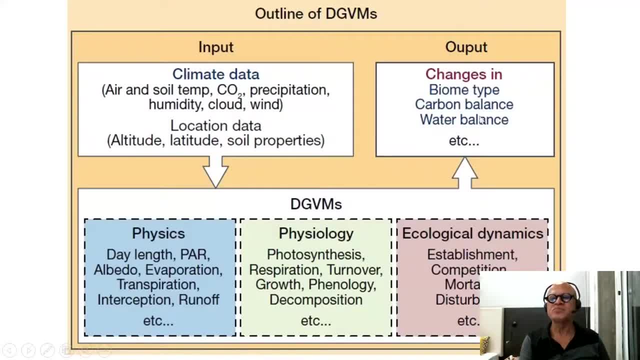 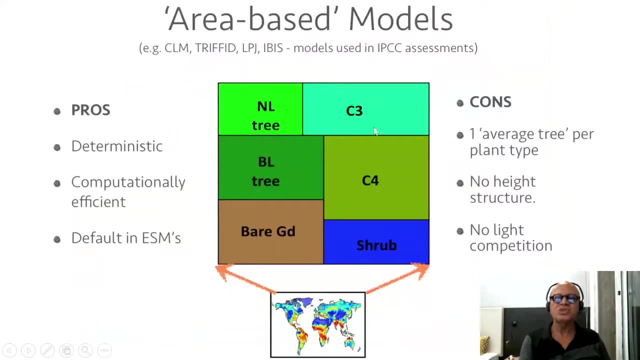 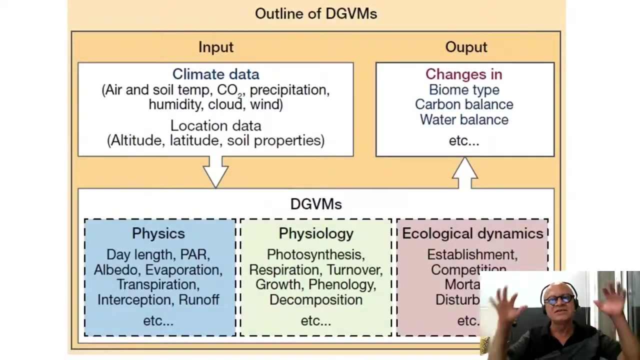 climate data, location data, changes in biome types, carbon balance, water balance and so on, as the outputs going through the physics, the physiology and the ecological dynamics. So here you can in fact do competitions between C3 and C4 plants, with climate change as tropics expand.